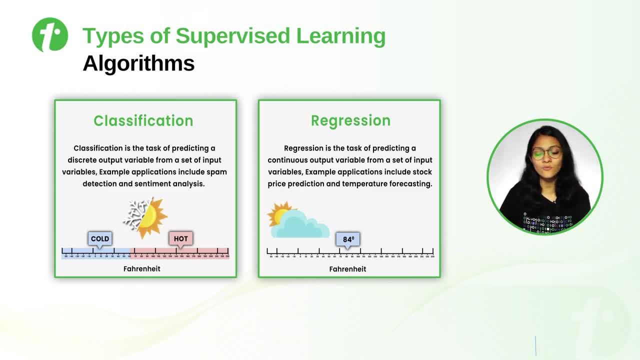 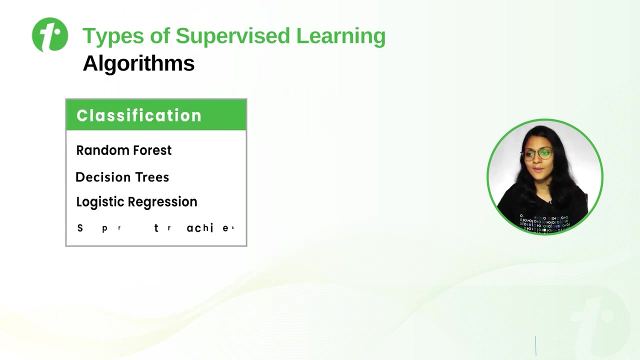 simple example: In case of classification, it is telling us whether the environment is hot or cold. That means we have only two categories as the output: hot and cold. In the case of regression, it is telling the exact value of the temperature, that it is 84 degree Fahrenheit. That means we have continuous value as the output. Random forest decision tree logistic regression support vector machines are the algorithms. that falls under the classification type problem. 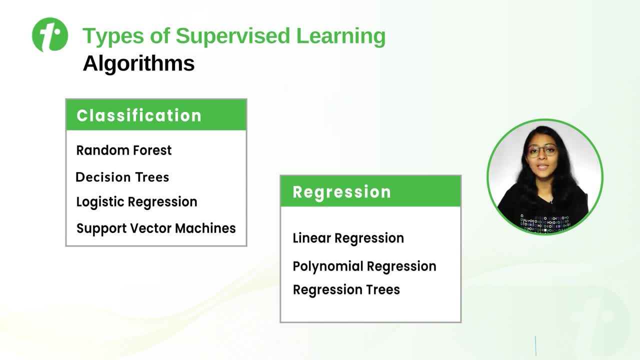 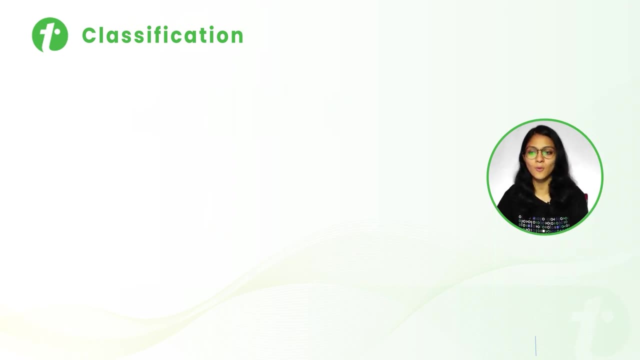 Linear regression, polynomial regression, regression trees are the algorithms that falls under the regression type problem. We are going to discuss all these algorithms in detail in further videos, So stay tuned with the tutorials point. Now let's discuss about the classification type problem with an example. We have two types of features. First is independent feature and second is dependent feature. All the input data that we provide to the model to predict some output are called input data. 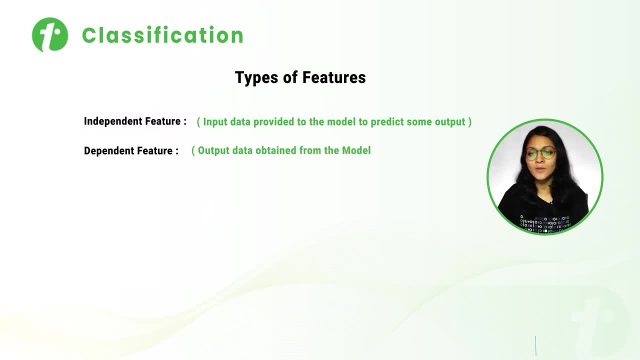 Independent features and the output that we obtain from the model are called dependent features. In this particular case, the number of hours for sleep, for playing games and for study are the independent features and the output- whether the student is going to pass or fail- is the dependent feature. We can observe here that we have only two categories in the output variable, That is, either the student is going to pass or fail the exam. 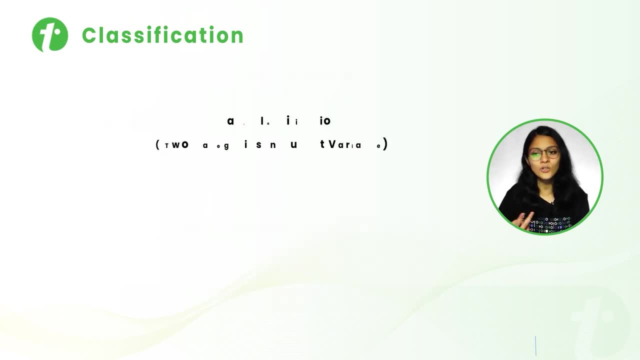 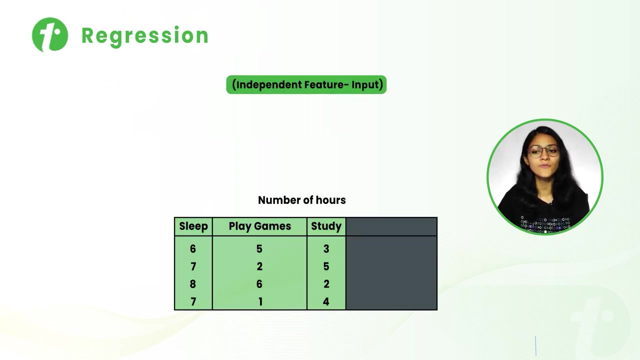 That means we have categorical output. If we have only two categories in the output variable, then it becomes binary classification, And if we have more than two categories, then it will become multi-class classification. Now, next, let's talk about regression type problem. In this case, again, the number of hours for sleep, playing games and study are the independent features and the max percentage obtained is output variable. 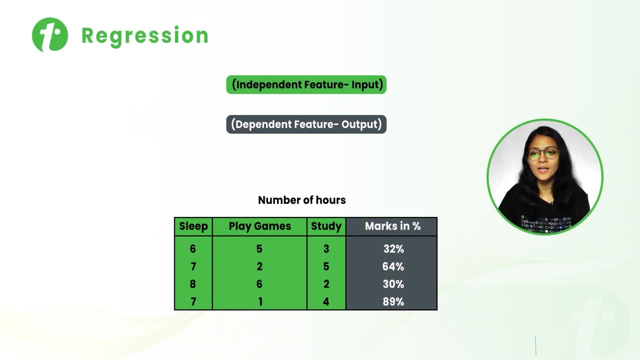 Now. next let's talk about regression type problem. In this case, again, the number of hours for sleep, playing games and study are the independent features and the max percentage obtained is output variable. We can observe here that we are getting the exact percentage marks of the students. That means we are getting some continuous value in the output variable. So this is a type of regression.